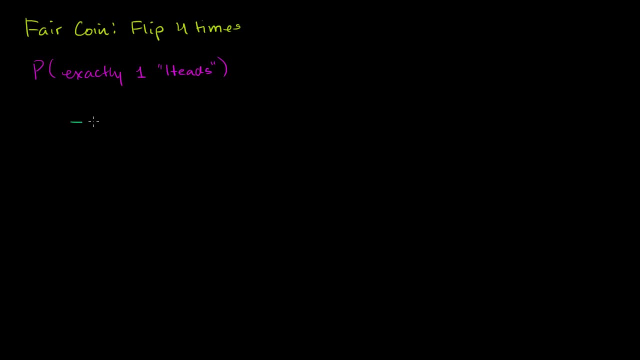 get four flips of a coin. So we're going to have one flip, then another flip, then another flip, then another flip. And this first flip has two possibilities: It could be heads or tails. The second flip has two possibilities: It could be heads or tails. 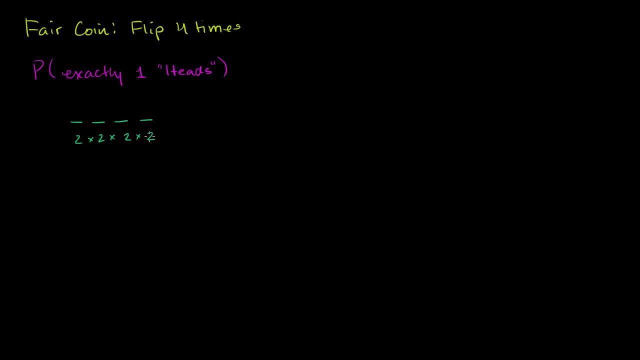 The third flip has two possibilities: It could be heads or tails. And the fourth flip has two possibilities: It could be heads or tails. So you have 2 times 2 times 2 times 2, which is equal to 16 possibilities. 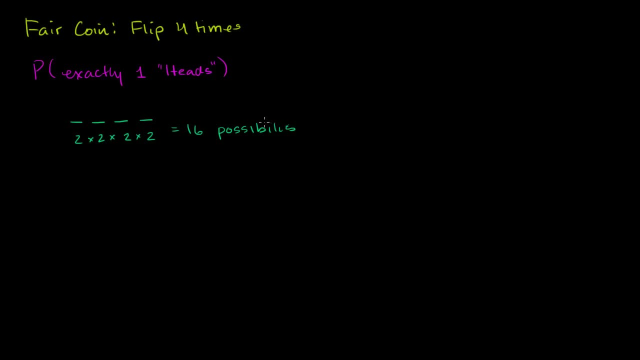 16 possible outcomes when you flip a coin, four times 16 possible outcomes And any one of the possible outcomes would be one of 16.. So if I were to just say the probability- and I'm just going to not talk about this- one heads. 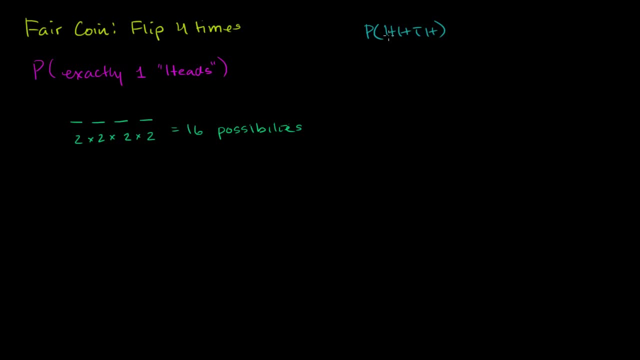 If I just take maybe this thing that has three heads right here, this exact sequence of events, This is the first flip, second flip, third flip, fourth flip, Getting exactly this. this is exactly one out of a possible of 16 events. 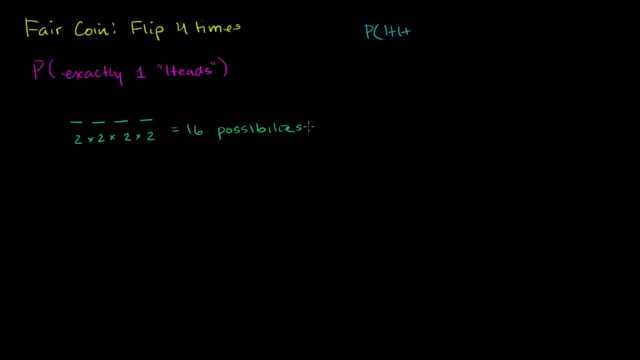 Now, with that out of the way, let's think about how many possibilities, how many of those 16 possibilities involve getting exactly one heads. Well, we could list them. You could get your heads. So this is equal to the probability of getting the heads in the first flip. 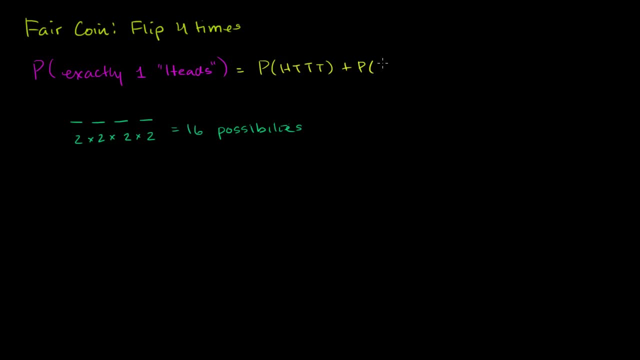 plus the probability of getting the heads in the second flip, Plus the probability of getting the heads in the third flip. Remember, exactly one heads, We're not saying at least one, exactly one heads. So probability in the third flip and then 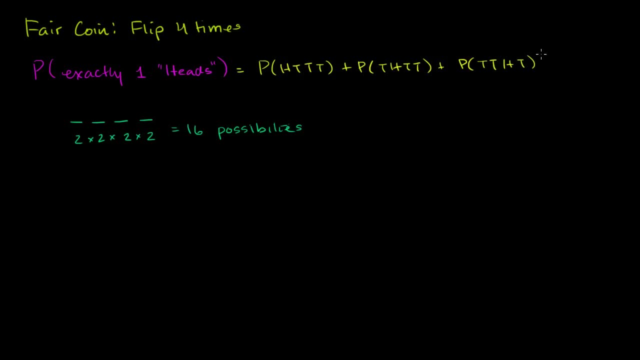 or the possibility that you get heads in the fourth flip Tails, heads and tails, And we know already what the probability of each of these things are. There are 16 possible events, and each of these are one of those 16 possible events. 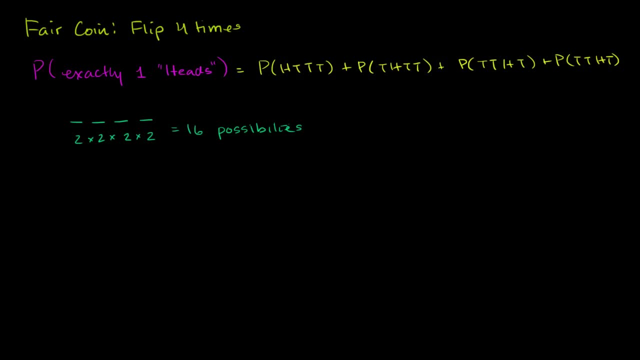 So this is the probability of getting the heads in the third flip. This is going to be 1 over 16,, 1 over 16, 1 over 16, and 1 over 16.. And so we're really saying the probability of getting exactly. 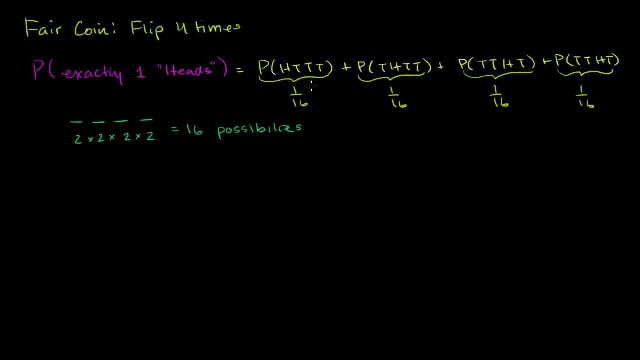 one, heads is the same thing as the probability of getting heads in the first flip, or the probability of getting heads in the first flip, or heads in the second flip, or heads in the third flip, or heads in the fourth flip, And we can add the probabilities of these different things. 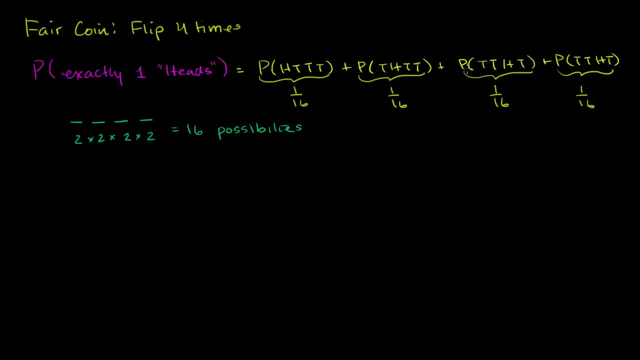 because they are mutually exclusive. Any two of these things cannot happen at the same time. You have to pick one of these scenarios, And so we can add the probabilities: 1 16th plus 1 16th plus 1 16th plus 1 16th. 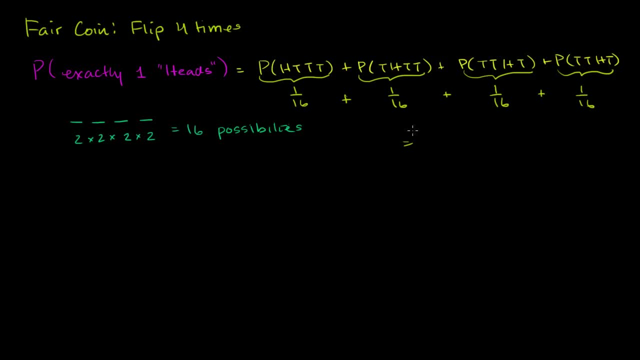 Did I say that four times? Well, assume that I did, And so you would get 4 16ths, which is equal to 1 fourth. Fair enough, Now let's ask a slightly more interesting question. Let's ask ourselves the probability. 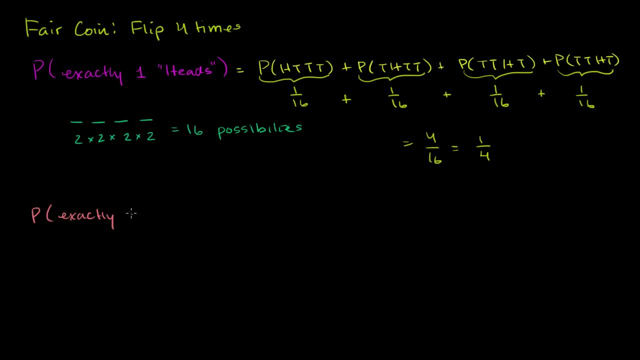 of getting exactly two heads, Exactly two heads. And there's a couple of ways we can think about it. One is just in the traditional way, And let's just look at the number of possibilities and of those equally likely possibilities, And we can only use this methodology. 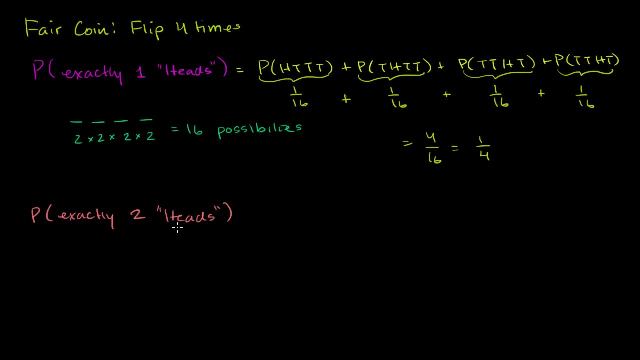 because it's a fair coin. So how many of the total possibilities have two heads of the total of equally likely possibilities? So we know there are 16 equally likely possibilities. How many of those have two heads? So I've actually Ahead of time. 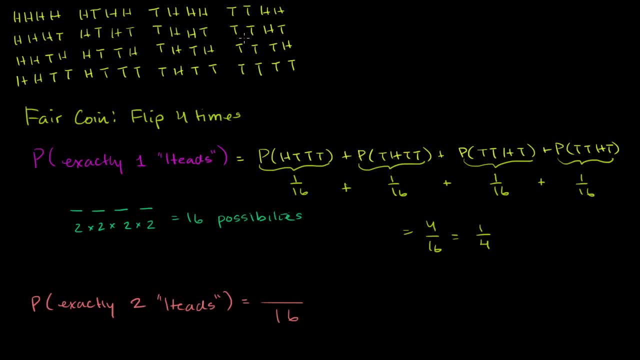 So we save time. I've drawn all of the 16 equally likely possibilities, And how many of these involve two heads? Well, let's see, This one over here has two heads. This one over here has two heads. This one over here has two heads. 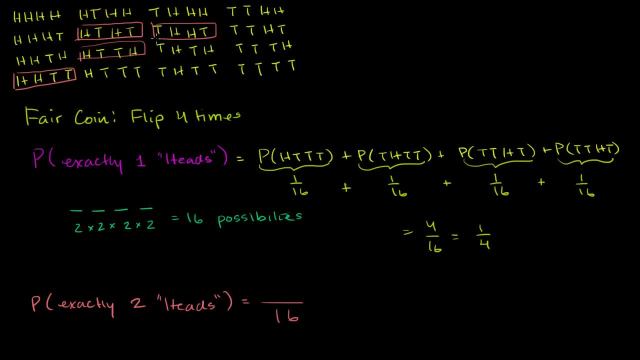 Let's see: This one over here has two heads, And this one over here has two heads, And then this one over here has two heads And I believe we are done after that. So if we count them, 1,, 2,, 3,, 4,, 5,, 6 of the possibilities. 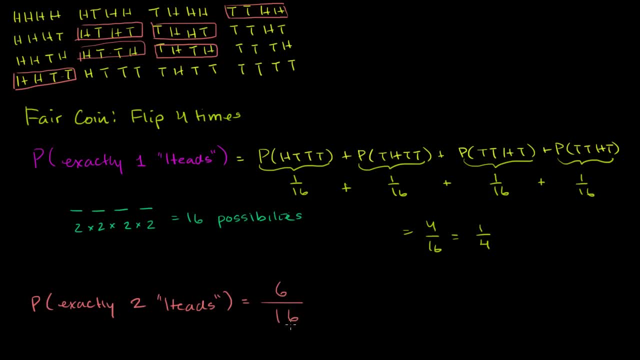 have exactly two heads. So 6 of the 16 equally likely possibilities have two heads. So we have a 3 eighths chance of getting exactly two heads. Now, that's kind of what we've been doing in the past, But what I want to do is think about it in a way. 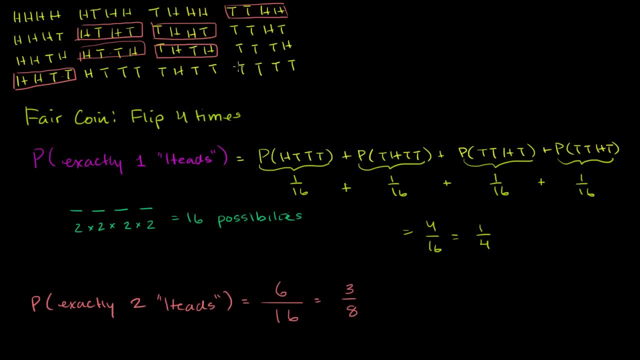 so we wouldn't have to write out all the possibilities. And the reason why that's useful is we're only dealing with four flips now, But if we were dealing with 10 flips, there's no way that we could write out all the possibilities like this. 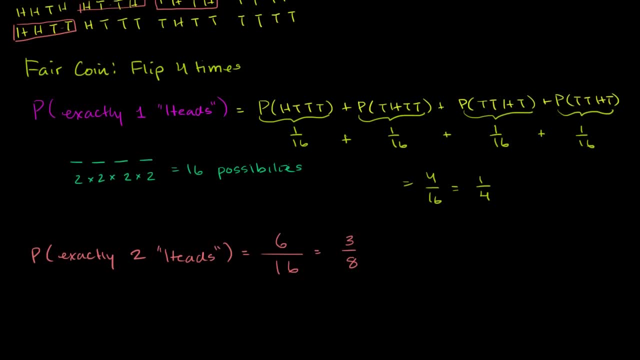 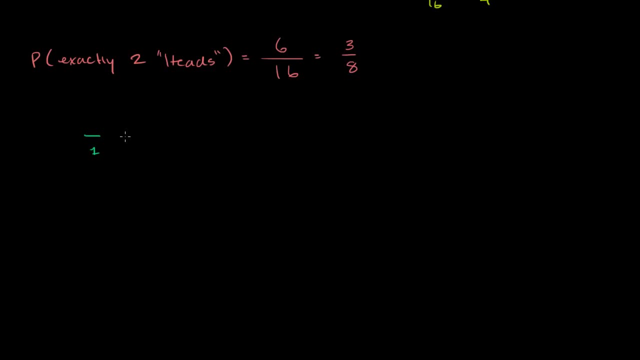 So I really want a different way of thinking about it. And the different way of thinking about it is, if we're saying exactly two heads, you can imagine we're having the four flips: Flip 1,, flip 2,, flip 3,, flip 4.. 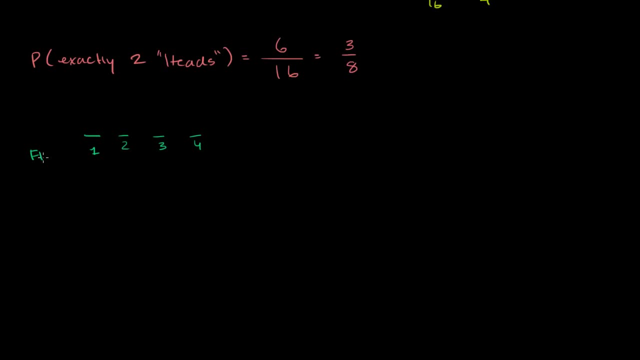 So these are the flips, or you could say the outcome of the flips, And if you're going to have exactly two heads, you could say: well, look, I'm going to have one head in one of these positions and then one head in the other position. 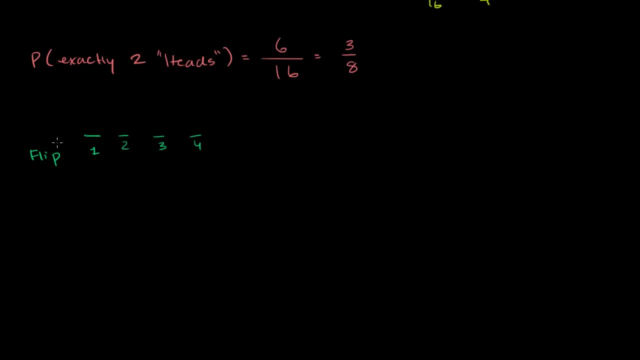 So how many? if I'm picking the first? so you could say: and I have kind of a heads 1, and I have a heads 2.. And I don't want you to think that these are somehow the heads in the first flip or the heads in the second flip. 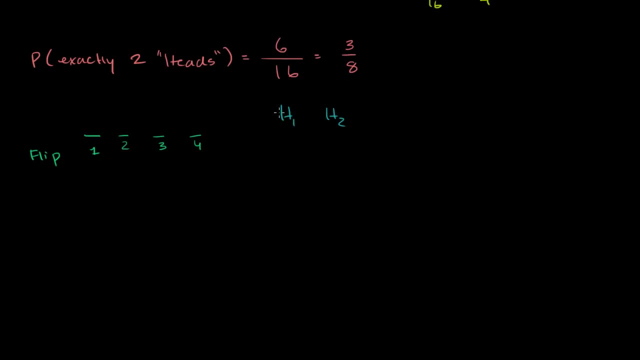 What I'm saying is we need two heads, We need a total of two heads in all of our flips, And I'm just giving one of the heads a name and I'm giving the other head a name, And what we're going to see in a few seconds. 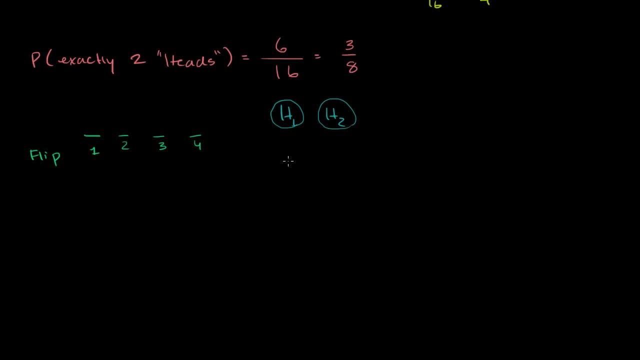 is that we actually don't want to double count. We don't want to count the situation, We don't want to double count this situation. Heads 1, heads 2, tails, tails, And heads 2, heads 1, tails, tails. 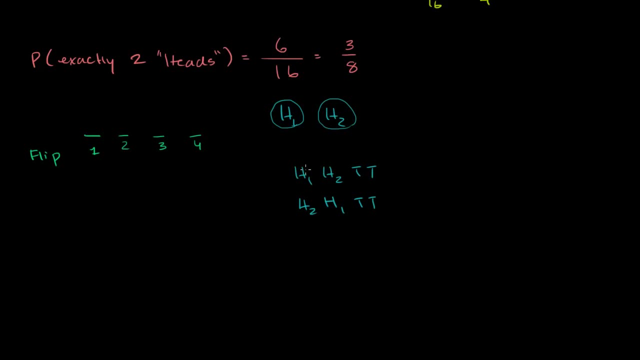 For our purposes these are the exact same outcomes, So we don't want to double count that and we're going to have to account for that. But if we just think about it generally, how many different spots, how many of different flips. 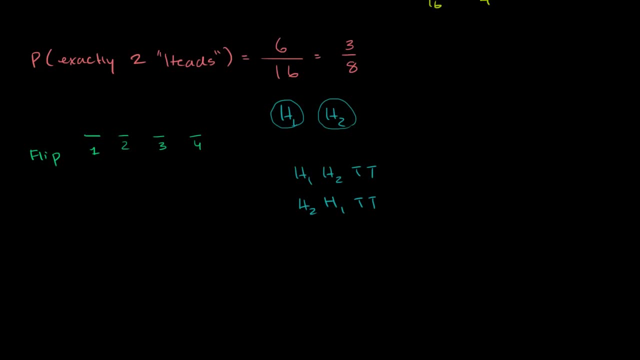 can that first head show up in? Well, there's four different flips that that first head could show up in. So there's four plus one, Four plus one. So there's four possibilities, four flips or four places that it could show up in. 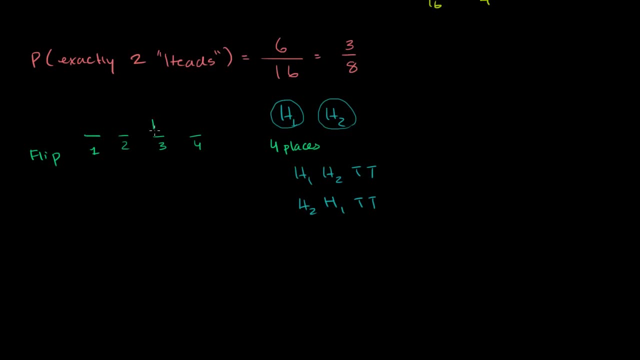 Well, if that first head takes up one of these four places- let's just say that first head shows up on the third flip- then how many different places can that second head show up in? Well, if that first head is in one of the four places, 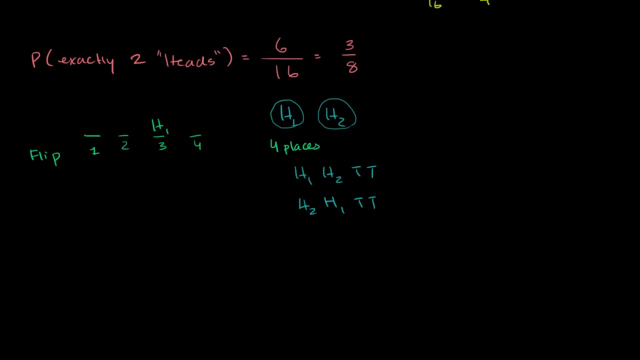 then that second head can only be in three different places. So that second head can only be in three different places, And so you know it could be in any one of these. It could maybe be right over there, any one of those three places. 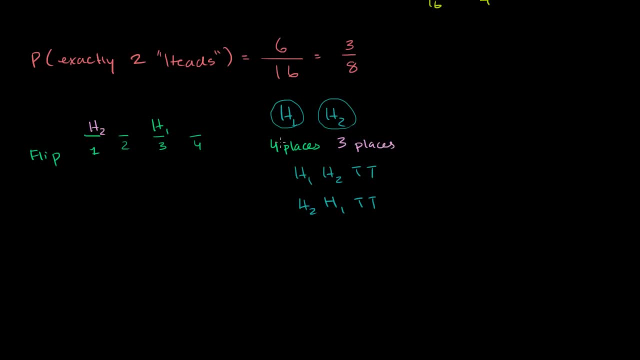 And so when you think about it in terms of the first- and I don't want to say the first head- head one. Actually, let me call it this way, Let me call it head A and head B. That way you won't think that I'm talking about the first flip. 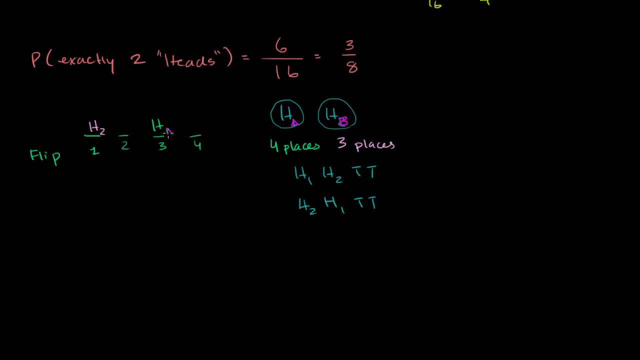 or the second flip. So this is head A and this right over there is head B. So, if you had a particular, I mean these heads are identical. These outcomes aren't different, But the way that you can think about it, 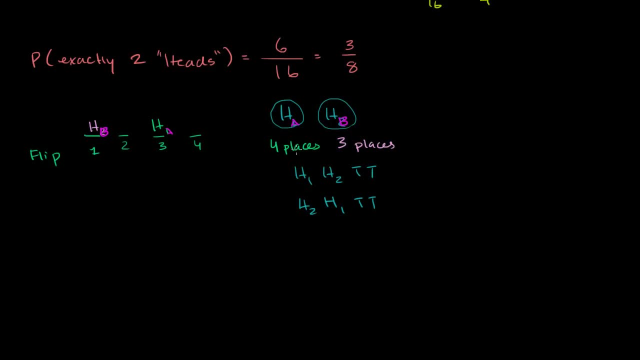 they aren't different, but the way we talk about it right now, it looks like there's four places that we could get this head in and there's three places where we could get this head in, And so if you were to multiply all of the different ways, 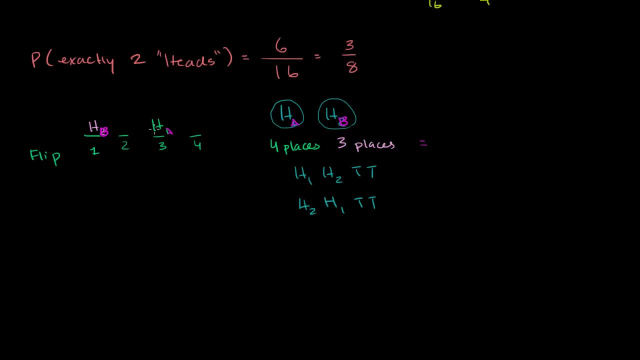 that you could get all of the different scenarios where this is in four different places and then this is in one of the three leftover places. you get 12 different scenarios, But there would only be 12 different scenarios if you viewed this This as being different than this. 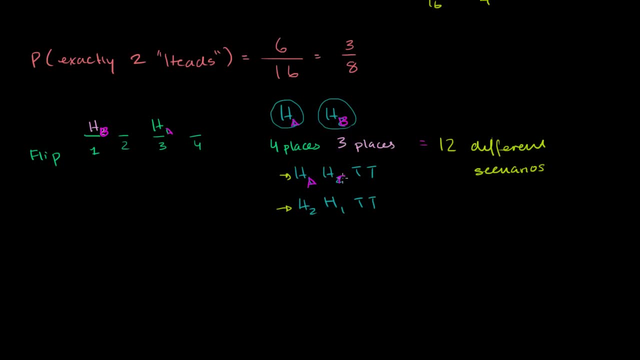 And let me rewrite it with our new. so this is head A, this is head B. this is head B. this is head A. There would only be 12 different scenarios if you viewed these two things as fundamentally different, But we don't. 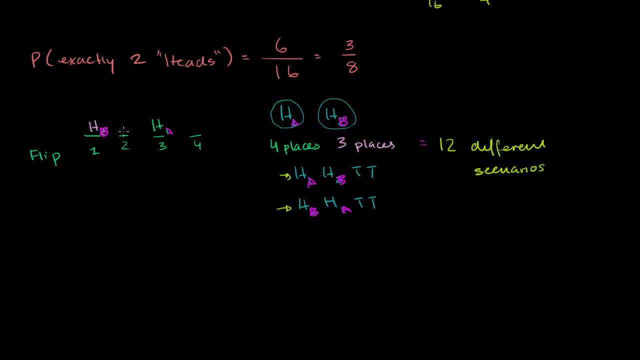 We're actually double counting because we can always swap these two heads and have the exact same outcome. So what you want to do is actually divide it by 2.. So you want to divide it by all of the different ways that you can swap two different things. 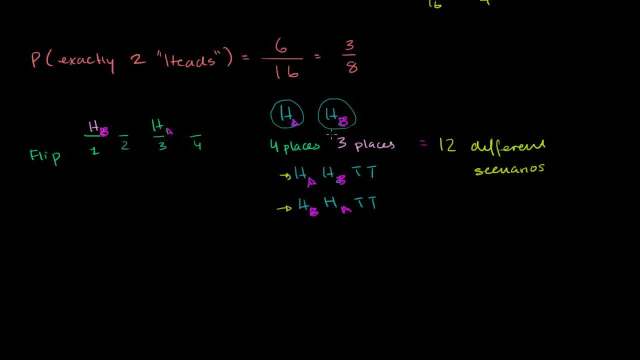 If we had three heads here, you would think about all of the different ways that you could swap three different things. If we had four heads here, it would be all of the different ways you could swap four different things. So there's 12 different scenarios. 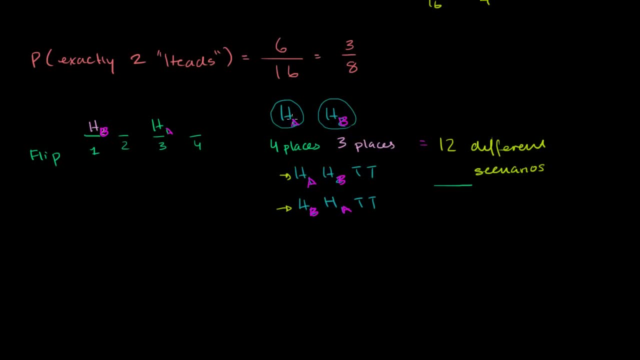 if you couldn't swap them. but you want to divide it by all of the different ways that you can swap two things. So 12 divided by 2 is equal to six different scenarios, fundamentally different scenarios, considering that you can swap them. 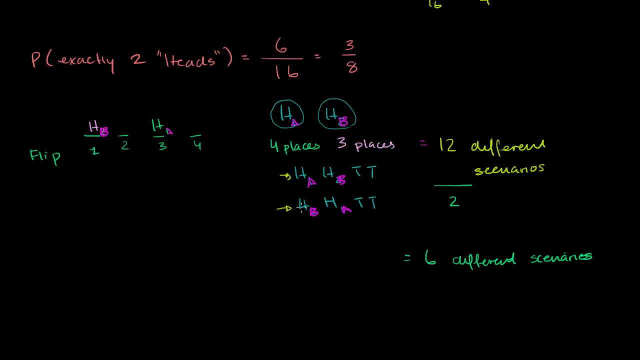 If you assume that That head A and head B can be interchangeable, that it's a completely identical outcome for us because they're really just heads. So there's six different scenarios and we know that there's a total of 16 equally likely scenarios.